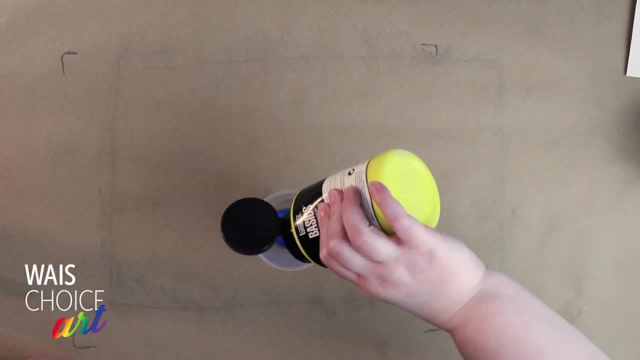 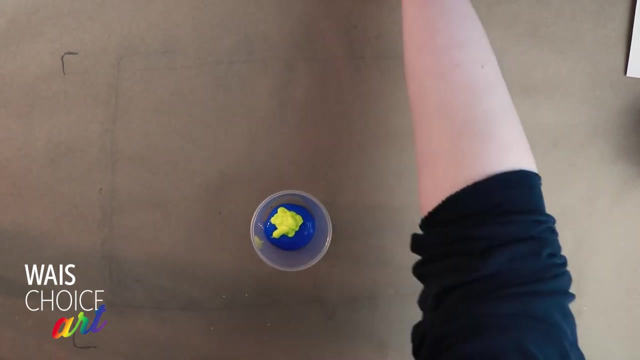 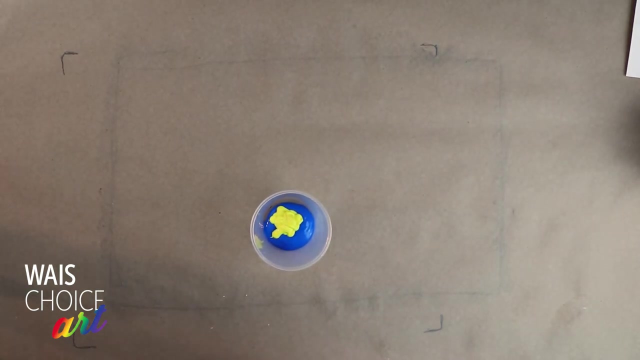 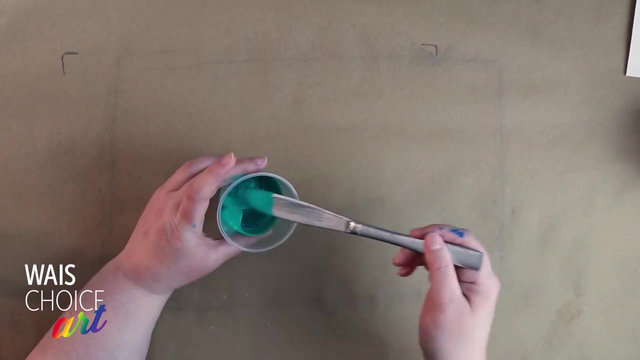 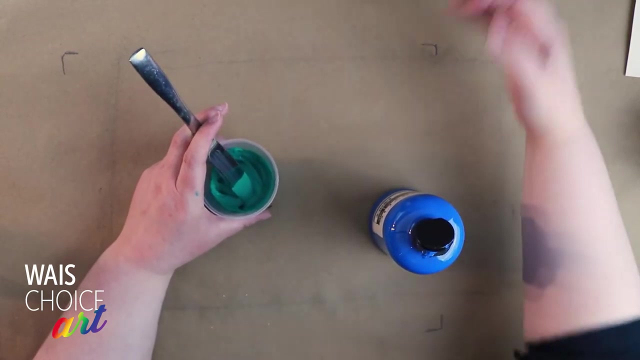 Alright, since I know this yellow is very transparent, I'm going to add a little bit of white right away, Just so I don't have to deal with that. Here we go. Alright, I have quite a bit of emerald green going on here. Let's add some more blue. 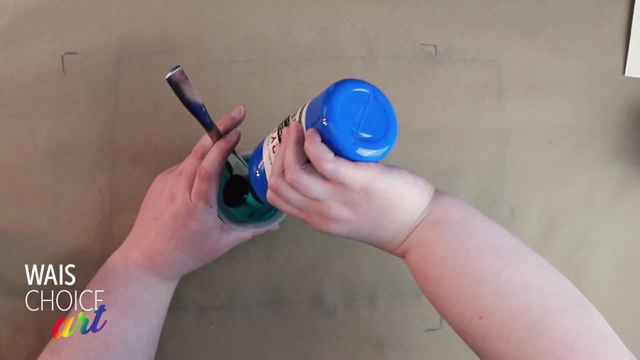 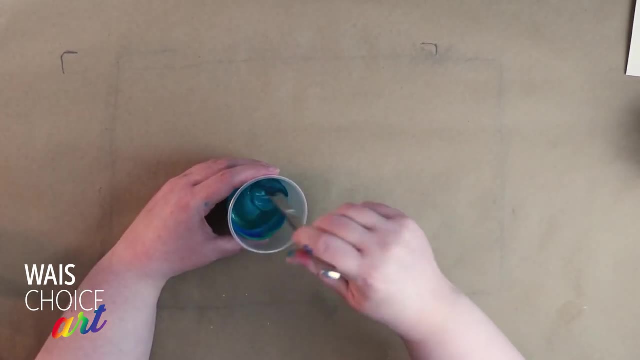 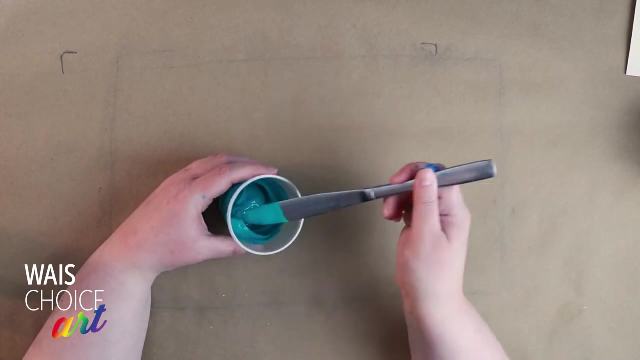 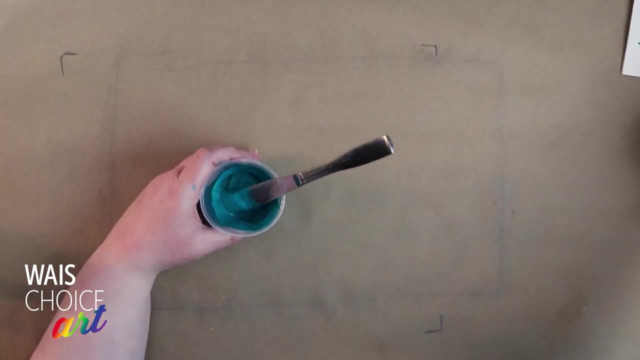 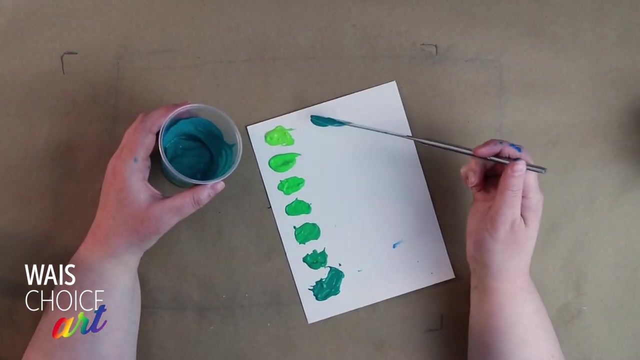 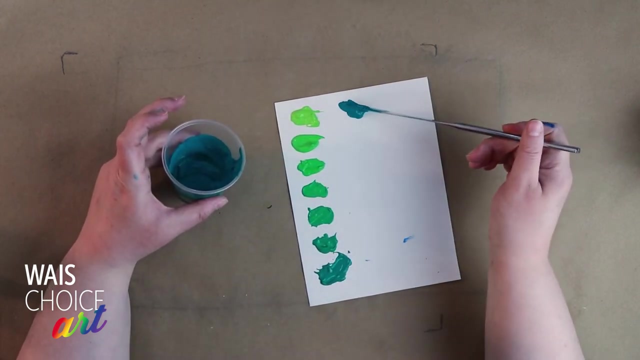 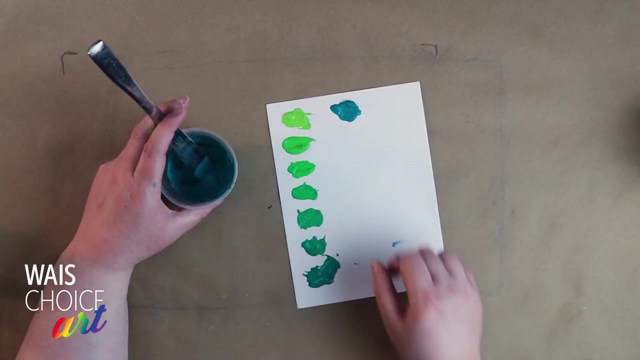 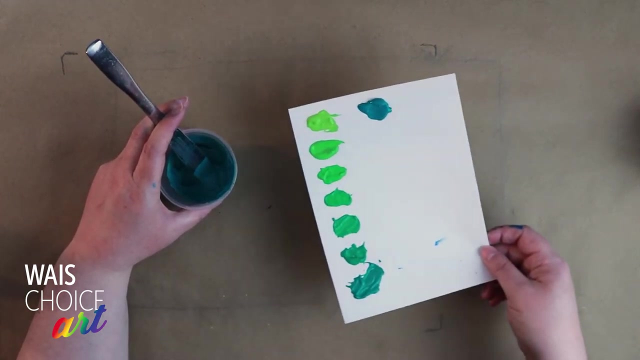 There we go, There we go. That's a decent deal, Alright. see the difference between the chartreuse we made and the green video, and now this Same two colors. Alright, let's see if we can make more of a turquoise. 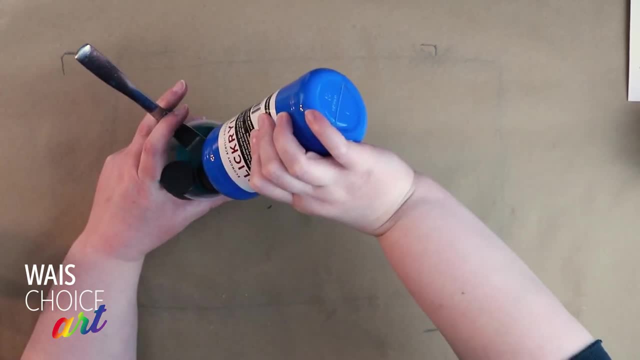 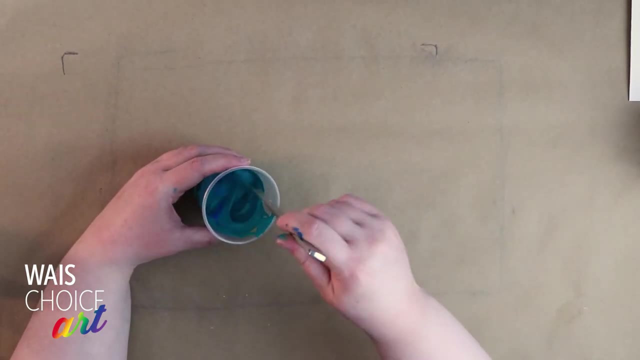 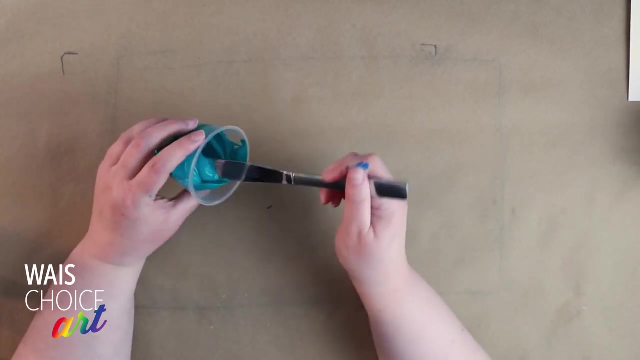 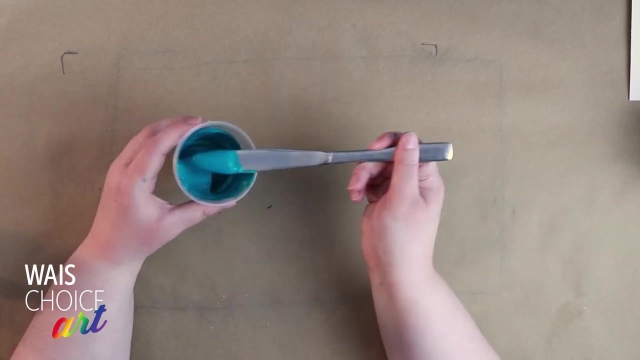 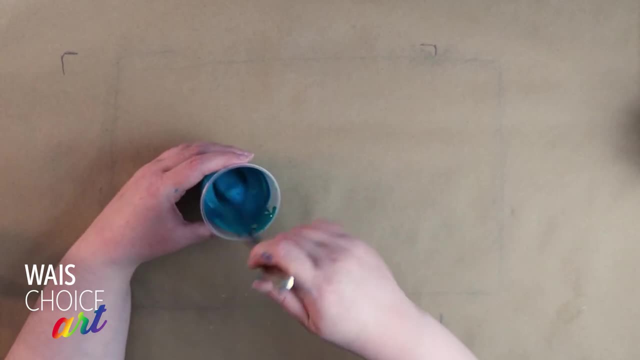 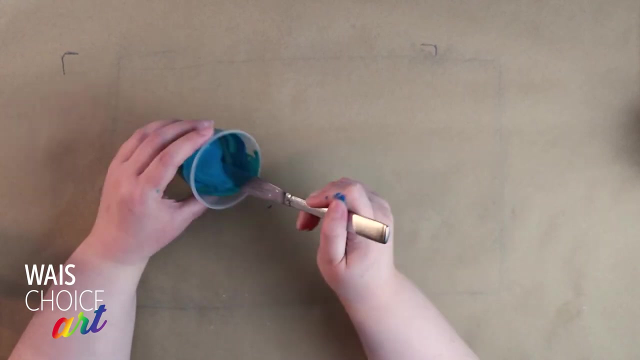 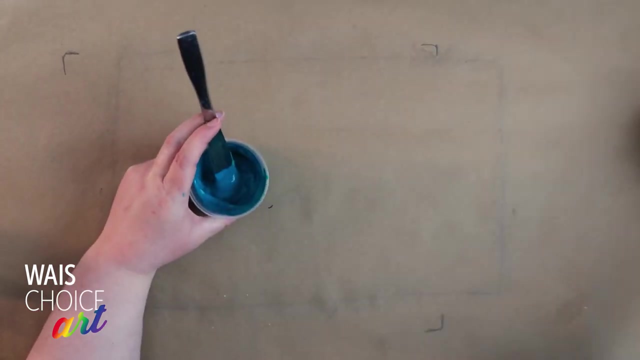 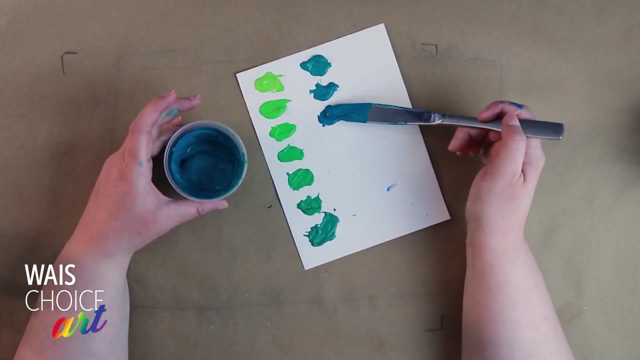 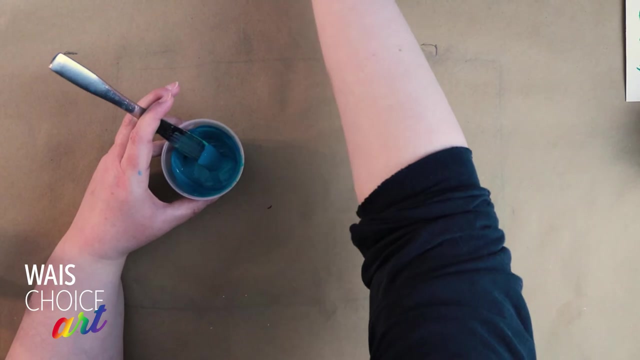 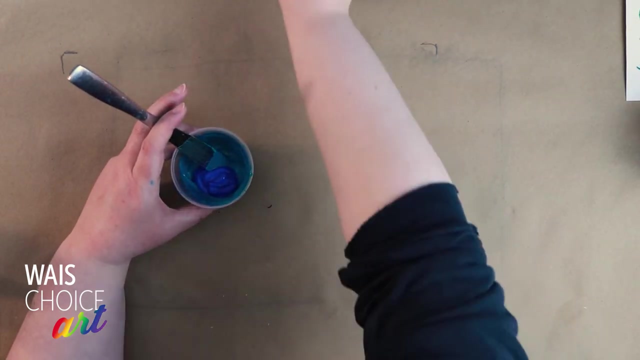 So let's go ahead and do that. That's a nice turquoise, Alright, let's see if we can do. aqua is hard. Let's see if we can do that. I'm going to take a little bit of white too. 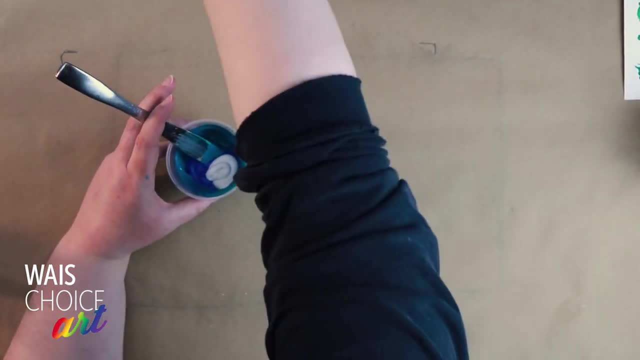 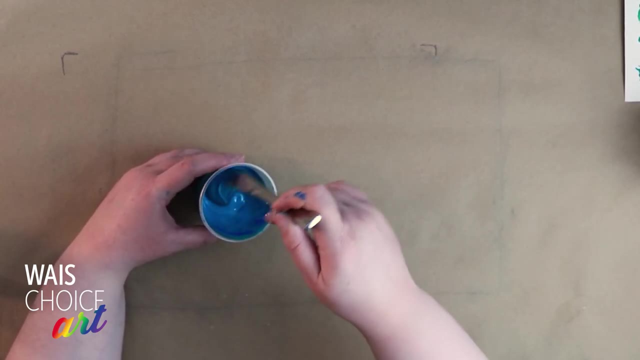 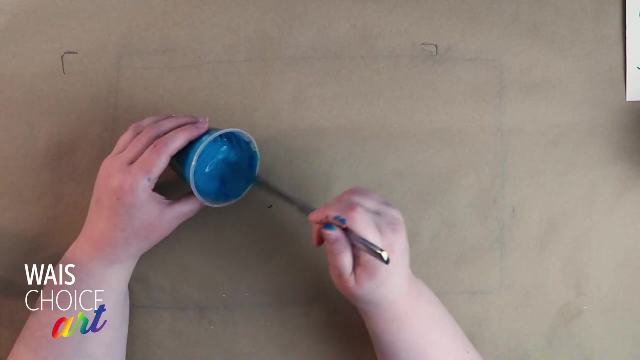 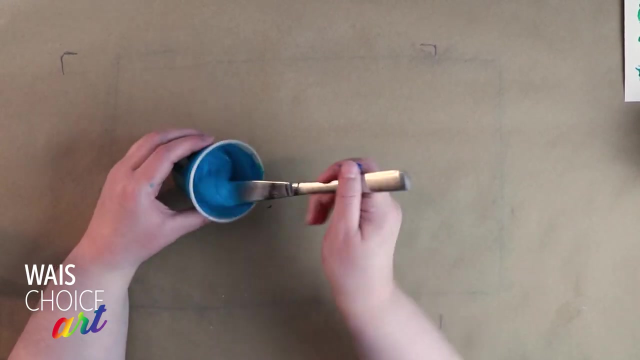 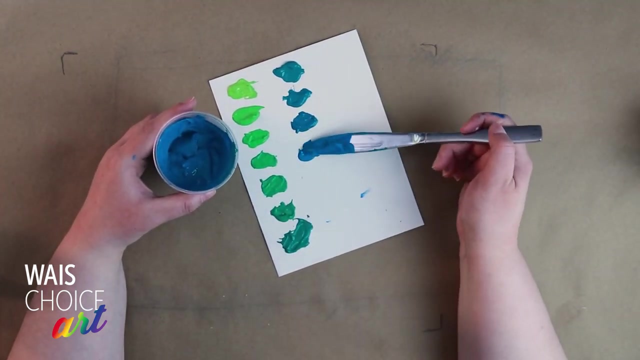 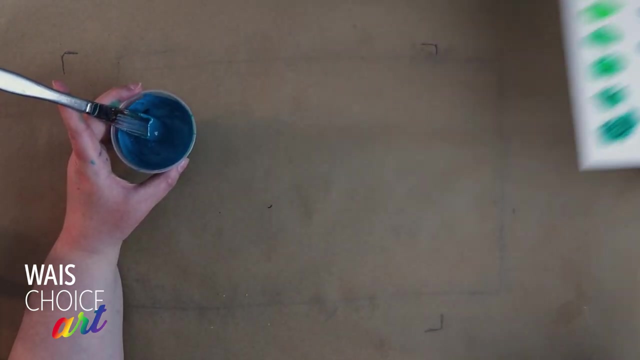 Let's see if we can do that. I don't know why. I seem to find the blues, the blue-green- is the easiest one to mix. Maybe I just like the color and they all look nice to me. It's actually kind of a nice light turquoise. 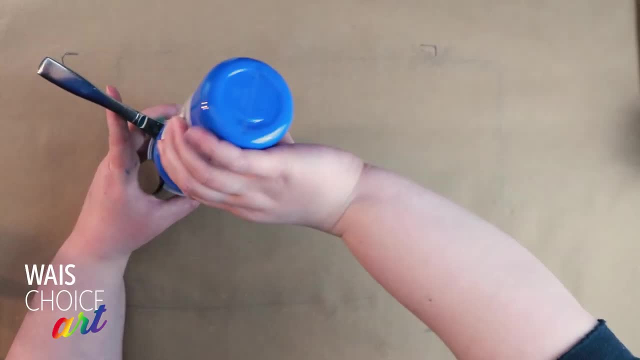 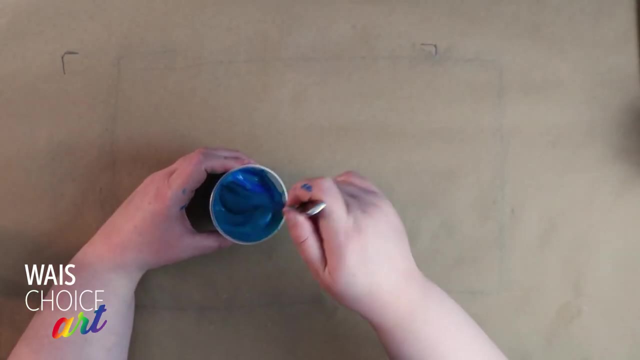 Let's do some more. blue Aqua is tough because it's kind of a bright color. If you don't have really bright pigments to start with, it's kind of weird. I just managed to get a light turquoise, Okay, Okay.